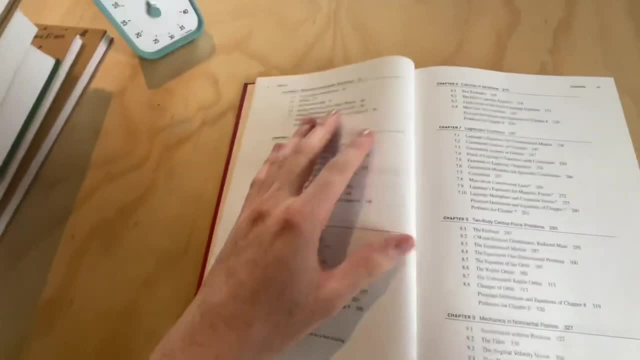 Chapter four is really where the difference starts, where you really move into a high level classical mechanics course. Chapter four is really where the difference starts, where you really move into a high level classical mechanics course. Chapter four is really where the difference starts, where you really move into a high level classical mechanics course. 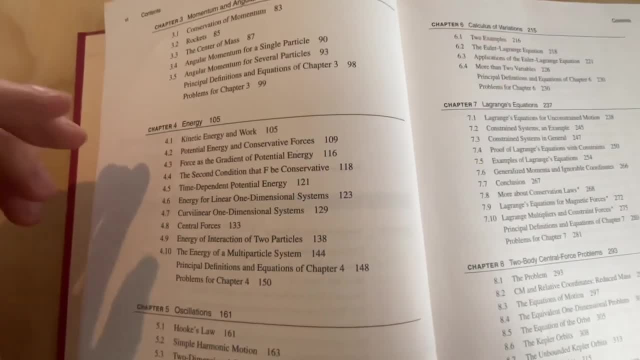 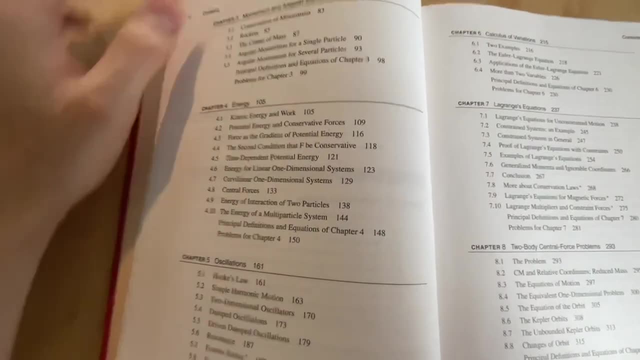 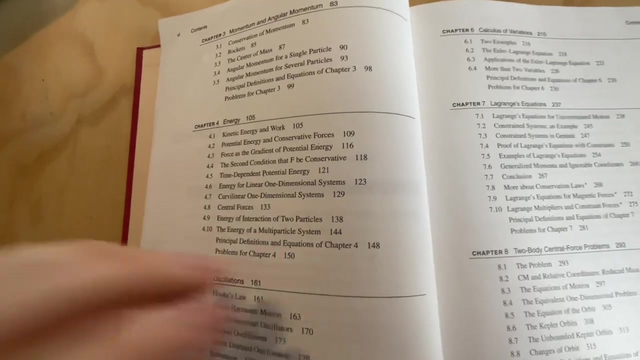 And the material here is really, really awesome. I absolutely love this chapter. It really connected a lot of the dots for me from other lower level classical mechanics classes. Talks a lot about path independence, deriving conservative forces from potential energies, that kind of stuff, The conditions for conservativeness- just really cool concepts. 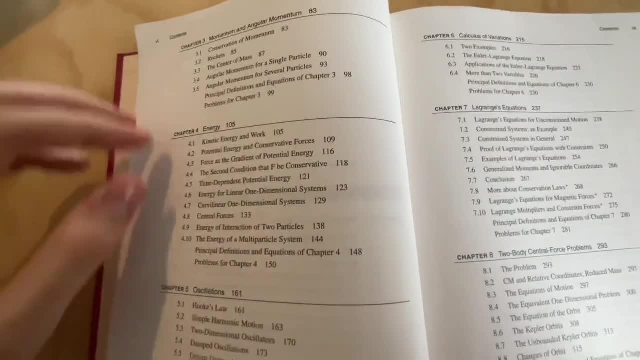 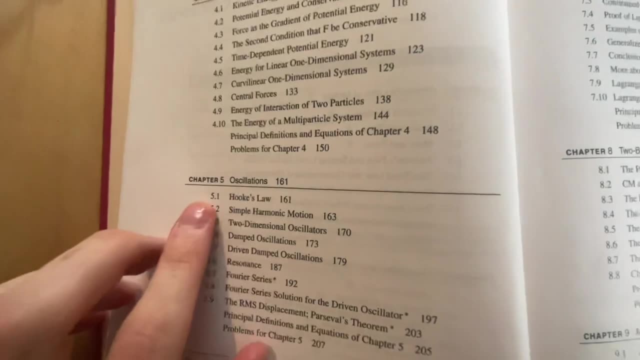 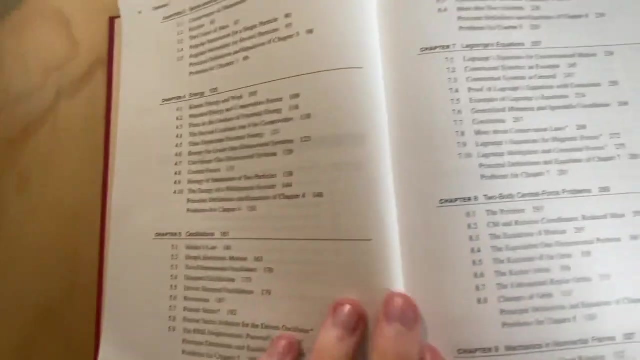 Also it uses a lot more mathematics that you usually don't see, or at least in lower level classes. So this chapter was really awesome. Oscillations just covers pretty much all the solutions to the differential equation for simple harmonic motion And it talks a little about damping and resonance and it even talks about 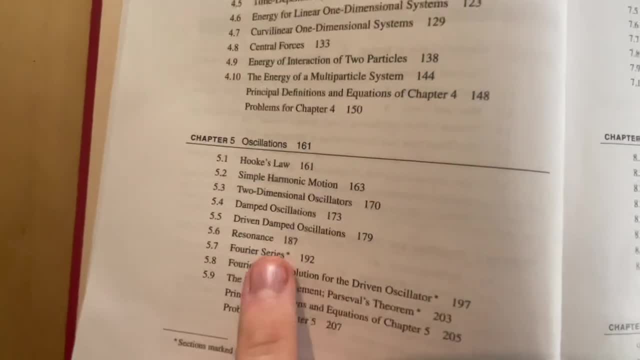 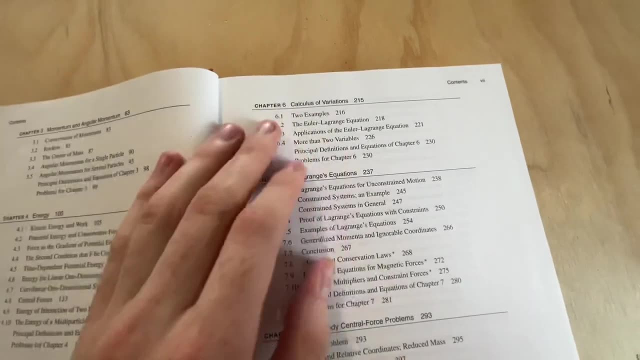 where is it Fourier series in here, which is a much higher level concept, So it was kind of cool to see it in there. Chapter six has a whole chapter dedicated to calculus of variations, which I thought this was really really good. 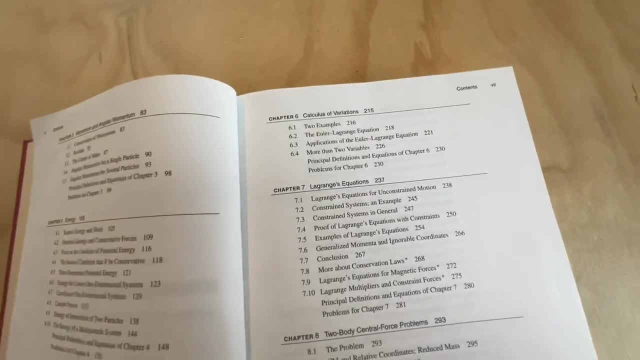 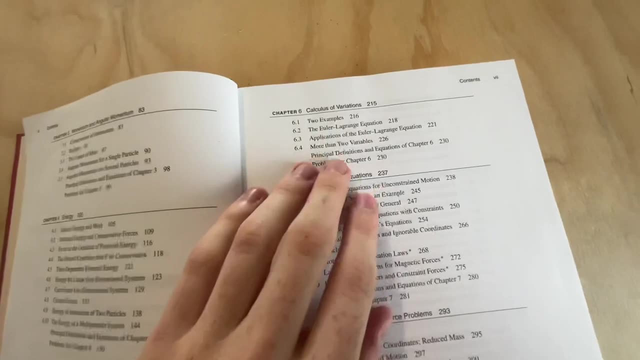 Taylor does an excellent job of deriving the Euler-Lagrange equations. I think it's really good, easy to follow and just really intuitive, Makes sense. He explains it really well All the topics in here. We've got, of course, the Euler-Lagrange equation. 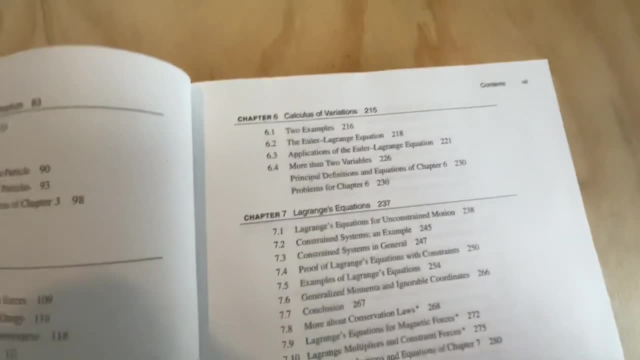 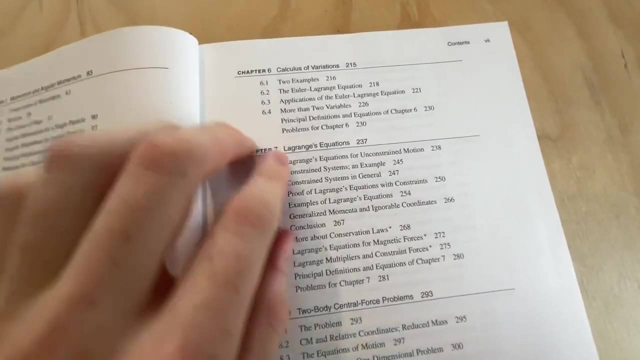 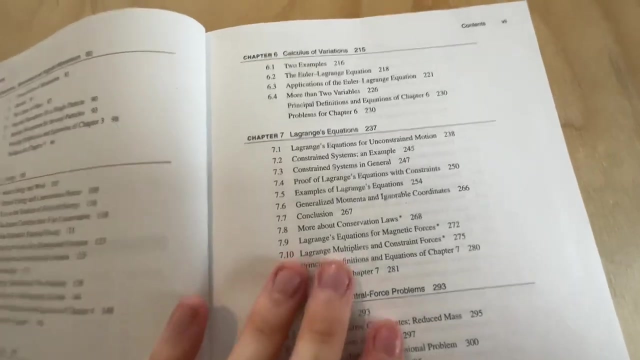 some applications, and it even talks about things like geodesics and Fermat's principle. And of course it's very natural just move into chapter seven of Lagrange's equations. The treatment here is excellent, excellent. i think it's honestly the best out of all the books i've read. um it just it's really. 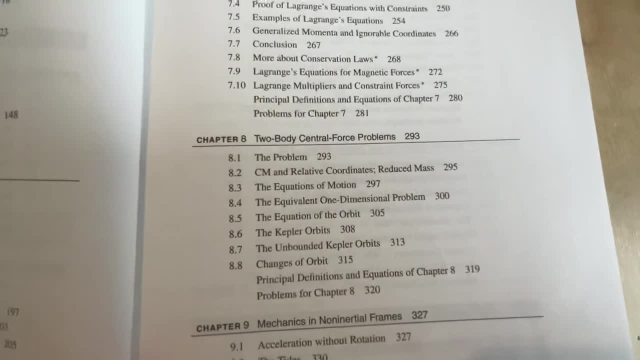 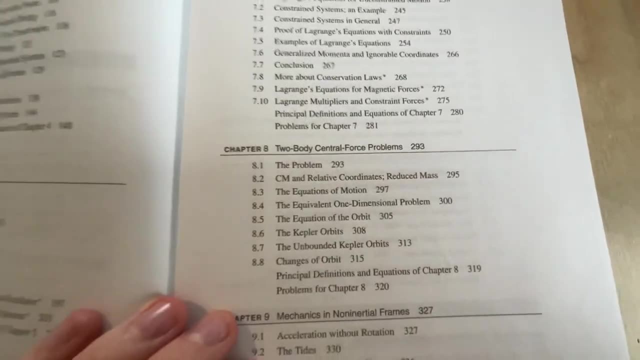 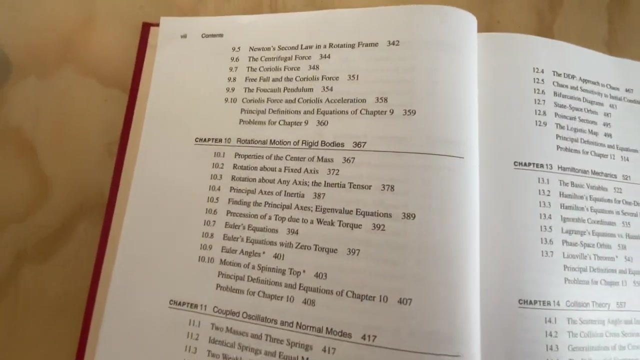 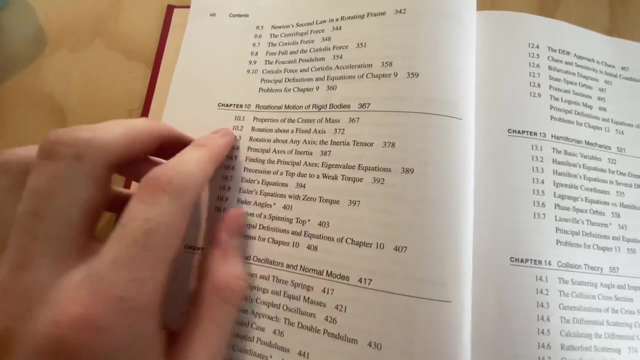 easy to follow, makes sense. and then of course you move on to two body central force problems. this is pretty natural continuation of lagrange's equations: mechanics and non-initial frames, rotational motion of rigid bodies. this section is very good. it's um probably one of the hardest, harder chapters in the book, but it covers everything well, i think. 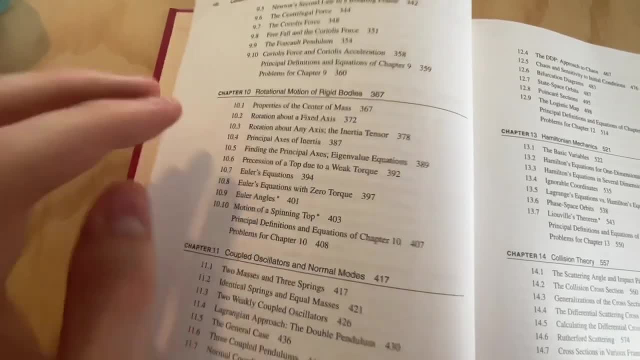 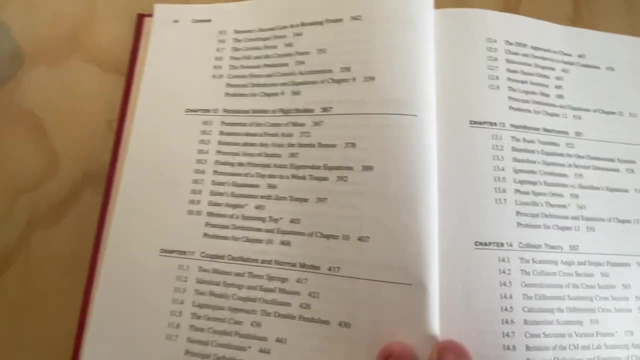 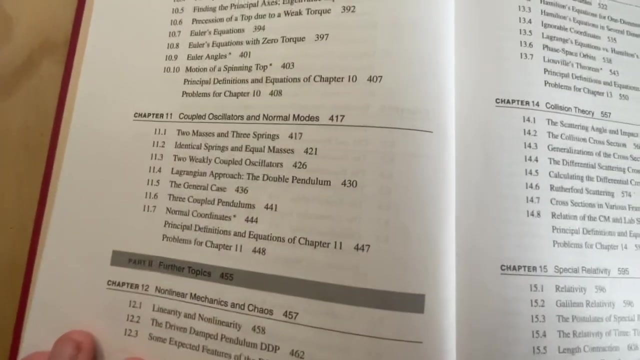 honestly, it is lacking, um, conceptually: why these things? these things are happening physically. all the math is there, but i think it's just lacking in that area: coupled oscillations and normal modes, mostly just treating the linear case, and then it moves on to further topics, first of which is non-linear mechanics and chaos. 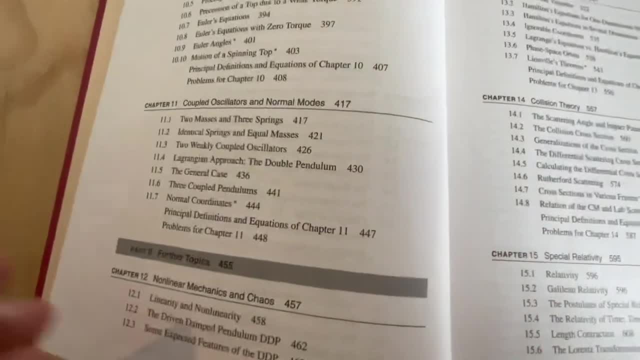 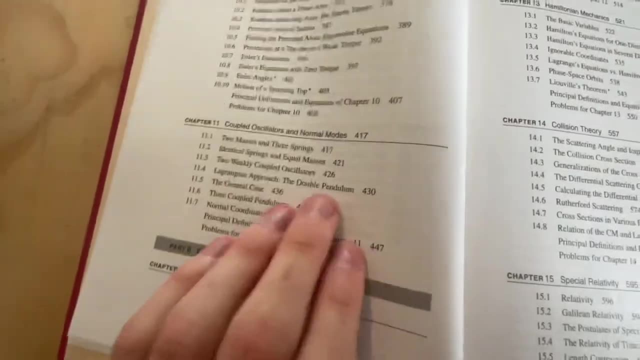 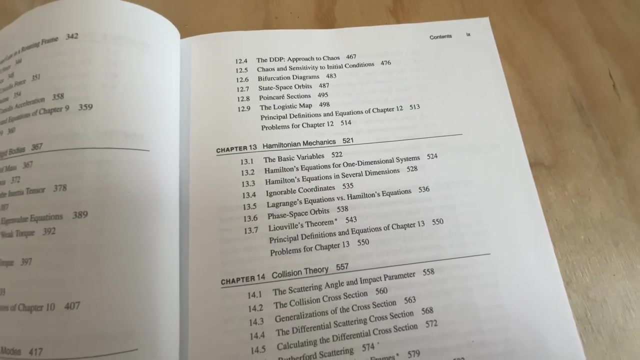 the. this is a really cool chapter because it's sort of filled in the gaps, especially in chapters like coupled oscillations and normal modes, where it doesn't talk about, um, the non-linear case. next we have hamiltonian mechanics. uh, honestly, this is a little bit underwhelming. 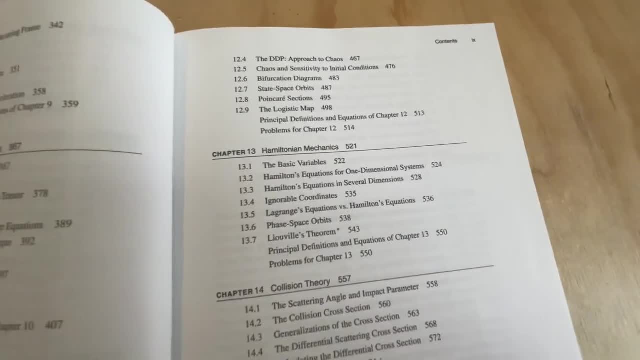 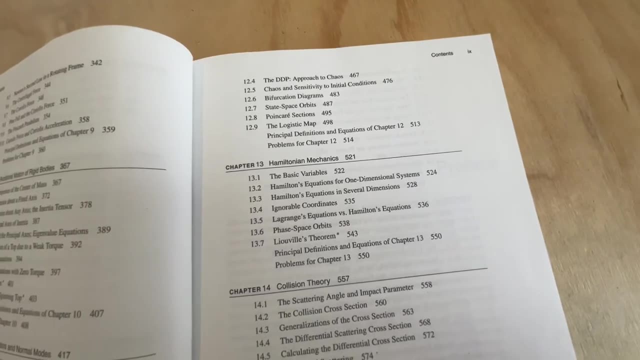 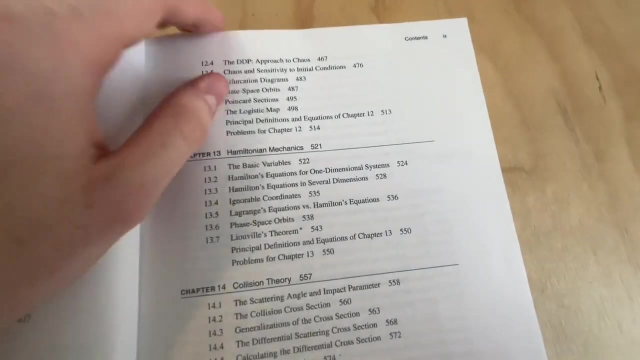 hamiltonian mechanics is, of course, another formalism of classical mechanics, but in this chapter it doesn't really even talk about why it's useful or what it's even used for, apart from perhaps discussing phase space and perhaps how that's geometrically better than than um state space. 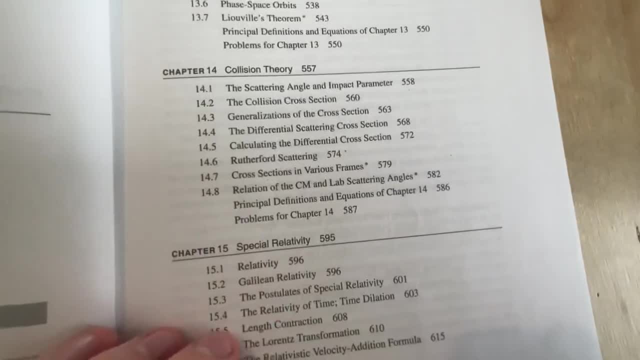 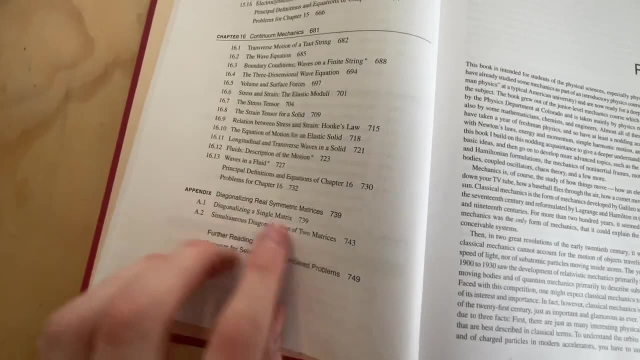 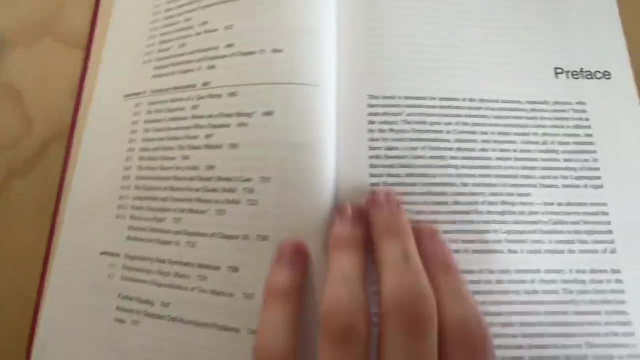 then we've got collision theory and special relativity, and then we finish off with continuum mechanics and we've got some appendix on linear algebra and some further reading. it also does have the answers to selected odd number problems, which is always nice, you know, for a book, to actually read the tables and stuff like that. so i'll just let that go at the end of this one. but i think it's really useful to know how to avoid problems of the sort, which is always nice, you know, from book to actual paper, for instance, we can use this problem a series of times as if we were going to put a string of numbers together and some of the models could be done in the same context, and we might not be able to do them if we were going to use more of them. but i think understanding the question is definitely a good idea. 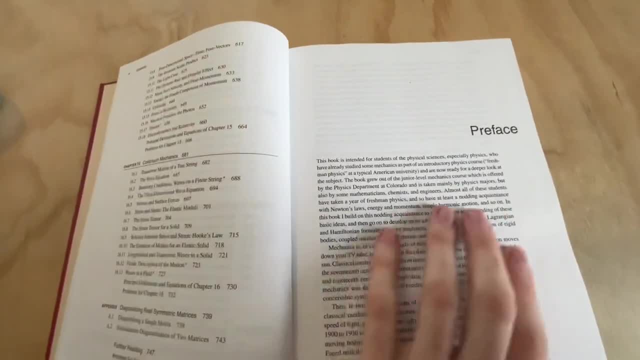 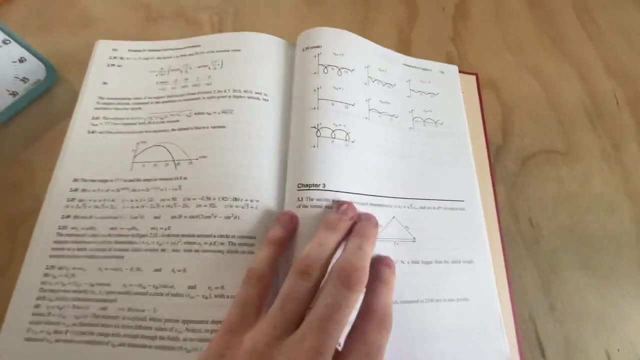 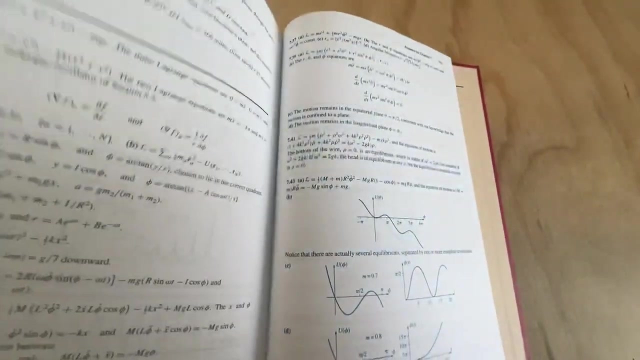 Which is always nice, you know, for a book to actually have some of the problem, some of the answers to the questions in the back, As you can see, solutions. A lot of them are quite partial as well, which is also kind of nice because it means that you have to do some of the work as well. 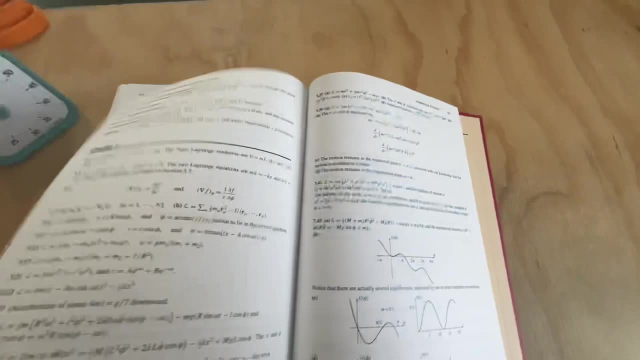 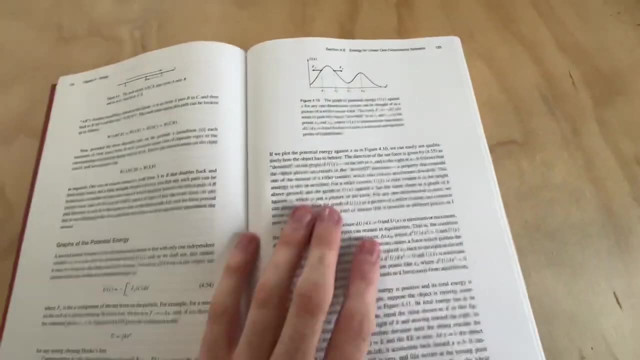 They're not full solutions. it will just give you an answer, So it doesn't show any of the working, But overall this book is just incredible. I think it's probably one of the best for undergrads taking classical mechanics. 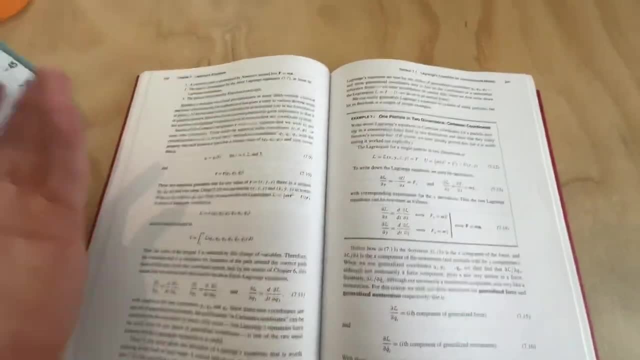 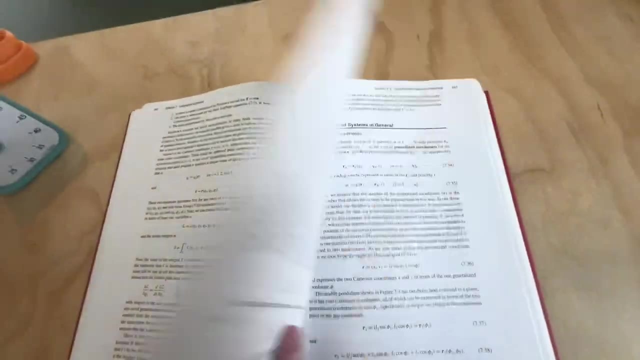 Probably something that it is lacking is that it doesn't really show how classical mechanics fits into physics really And how it relates to different areas of physics. Honestly, that would have been nice, because there are other books out there that do do exactly that. 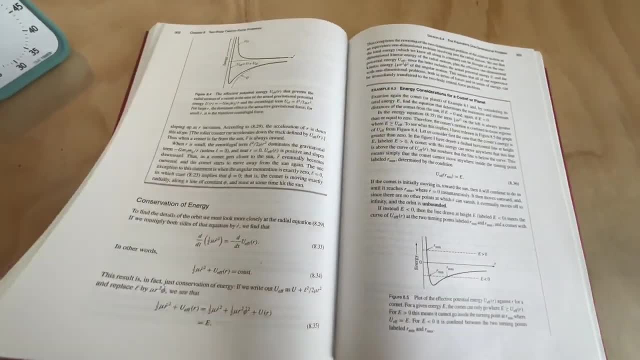 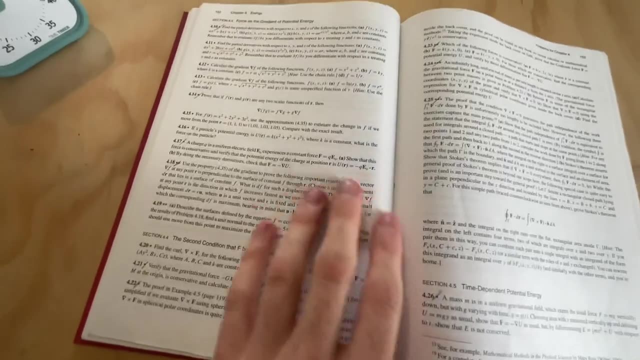 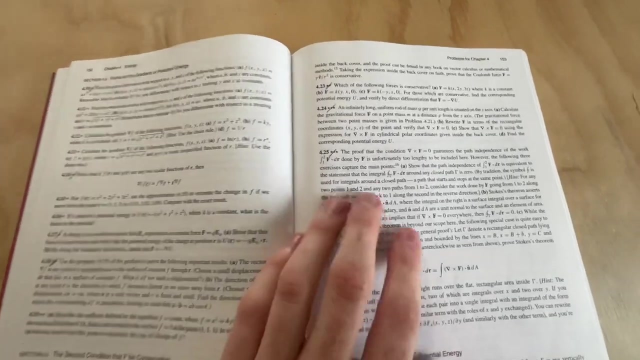 The readability on this thing is just incredible, and it doesn't sacrifice much rigour either for the readability. If I must make a word on some of the problems in this book, they can be quite bland, if I'm being honest. Some of them are more interesting, like here's one here that I found quite interesting. 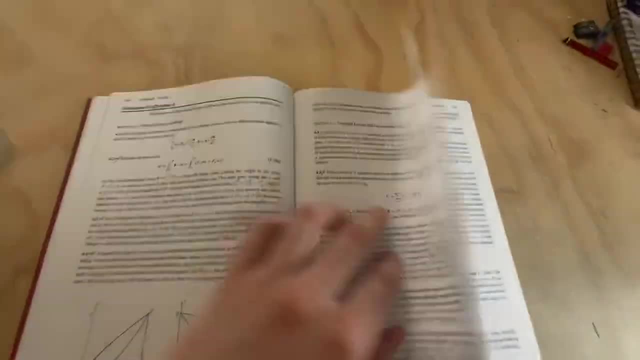 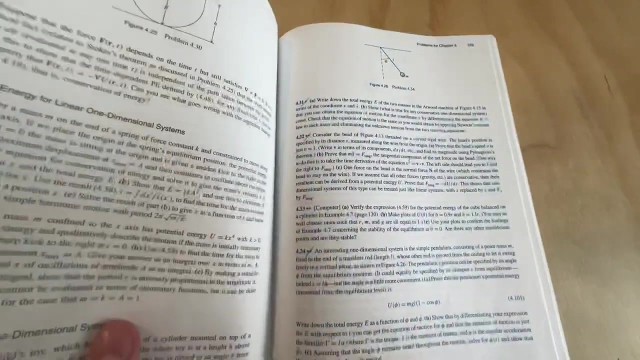 A lot of them can be quite bland and also repetitive- repetitive type of questions- But I mean they're pretty stable, They're pretty standard. really There's nothing. that's really too. They're not bad, they're just not exactly great. 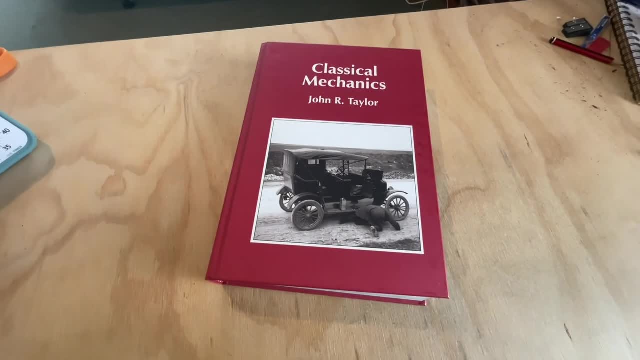 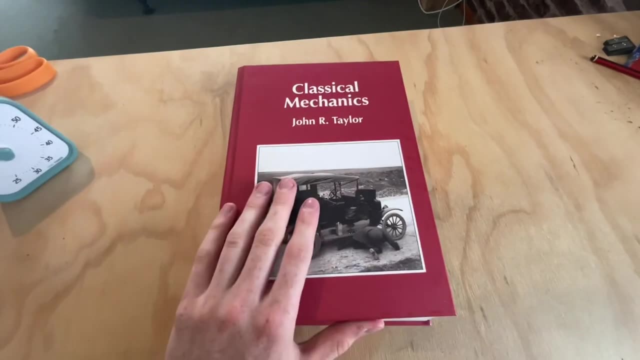 Some of them are interesting. So, overall, if you're thinking about picking up a book on classical mechanics at the undergraduate level and you've already had a solid class in classical mechanics and you want to take it further, this is probably the book for you. 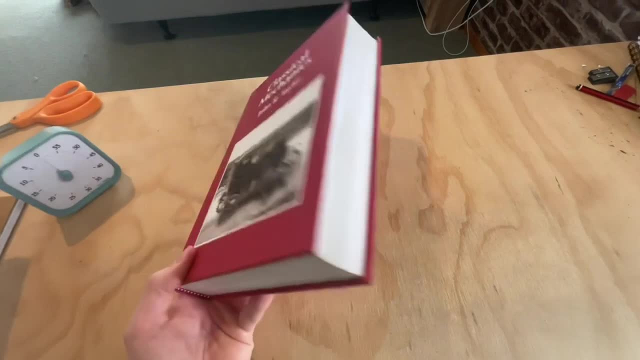 I 100% recommend it. Excellent print, excellent readability, Just all-round a good book. Thank you for watching. 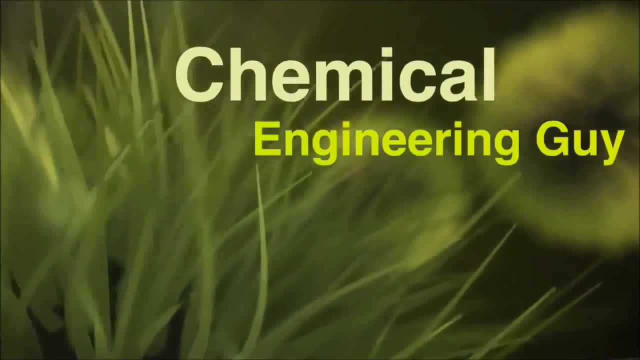 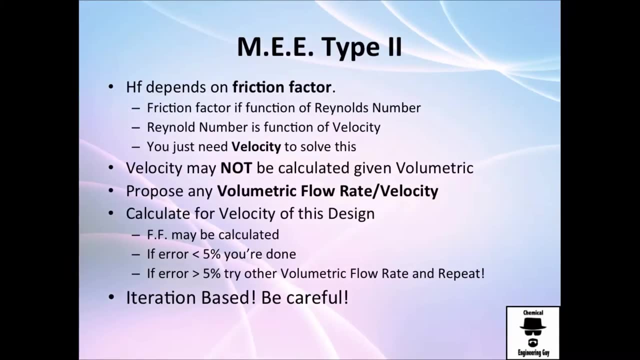 Now let's do an example of type number 2.. The thing here is that the energy loss due to friction depends on the friction factor and on the velocity head. The friction factor is function of Reynolds number, which at the same time is function of velocity. So we